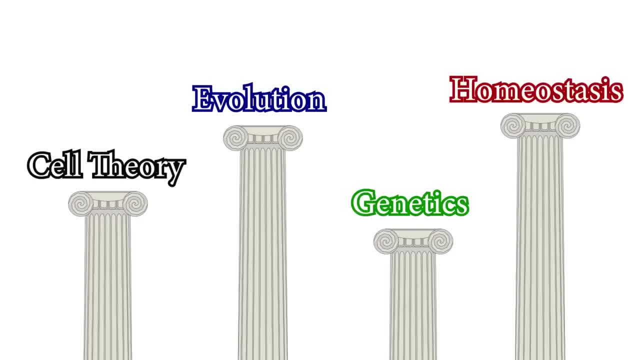 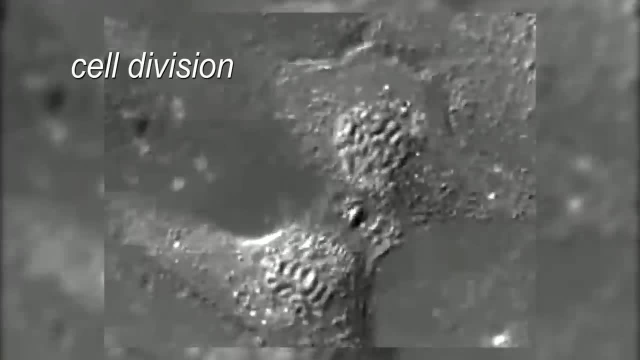 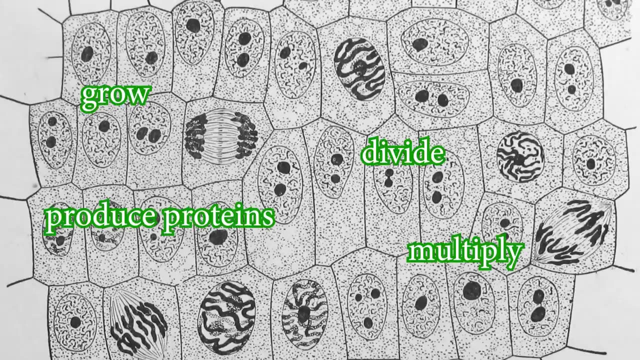 Cell theory, evolution, genetics and homeostasis. The cell theory implies that all living things are composed of cells and that all cells arise through cell division. These little building blocks are able to grow, produce proteins, divide, multiply and other cool stuff. 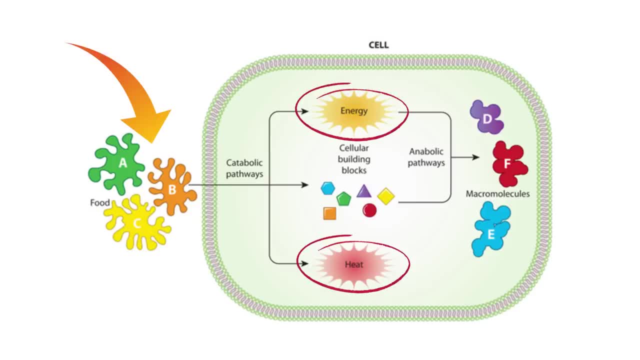 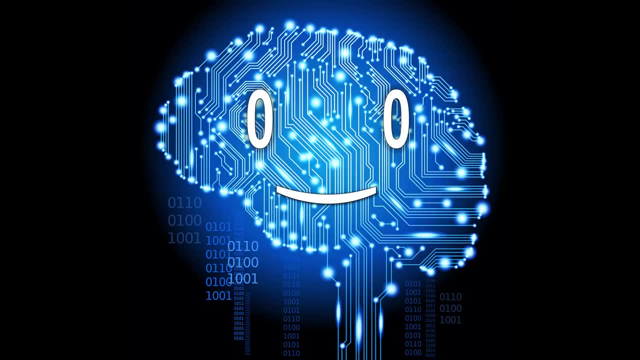 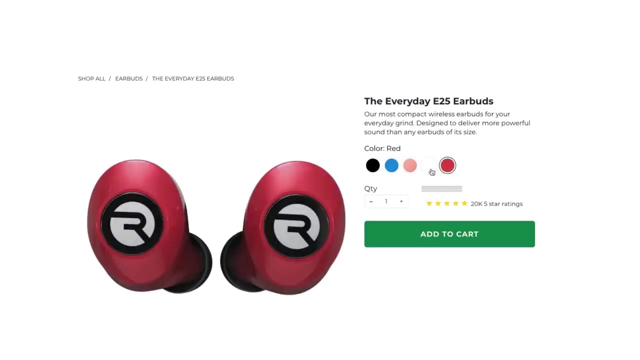 Thanks to metabolism, the process of converting food into energy and building materials. One of the cell's main function is to store data of the organism they are part of. Here comes genetics and our sponsor acknowledgement. Save 15% on your first order of the Raycon Wireless Earbuds by following this link, available in the description. 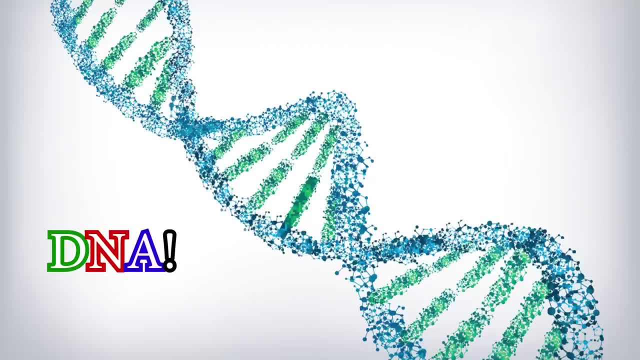 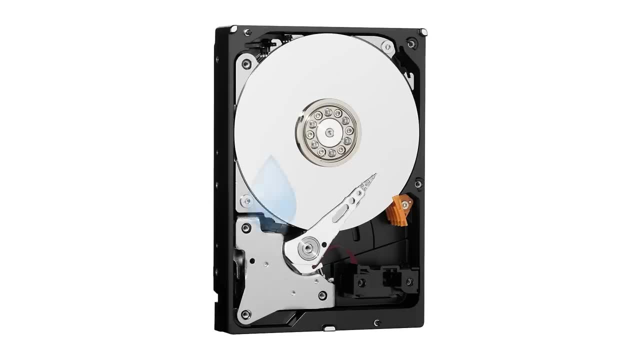 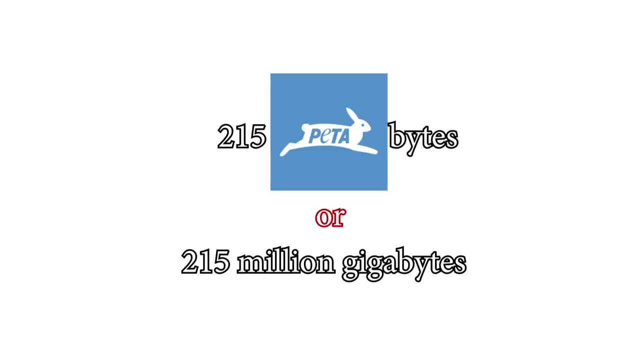 This data is stored in a special molecule called DNA. The unit of memory in the cell is called DNA. The unit of memory in a DNA molecule is the gene, which is way cooler than those pathetic bits of any hard drive. In a single gram of DNA you could store 215 petabytes or 215. 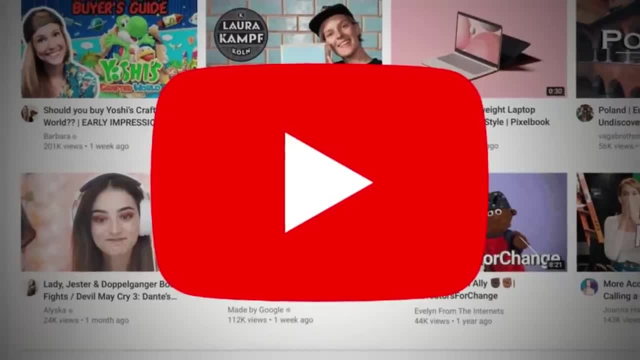 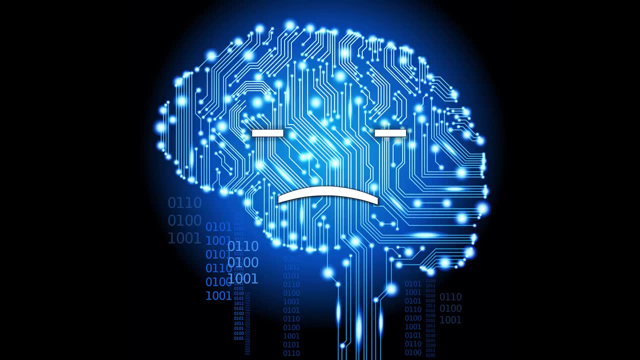 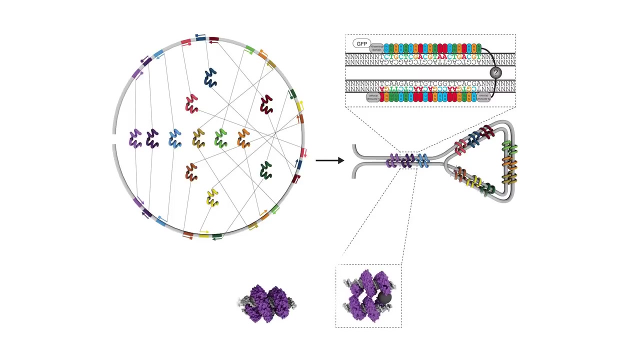 million gigabytes. For reference, to store all of the videos from YouTube, you would need 320 petabytes of storage, or a gram and a half of DNA. Still not enough for the new Call of Duty update. The information stored in the DNA is used for assembling. 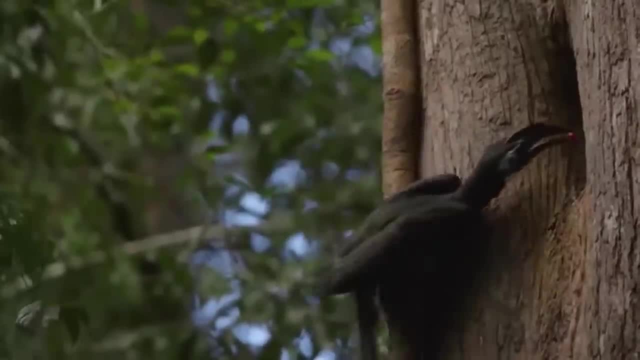 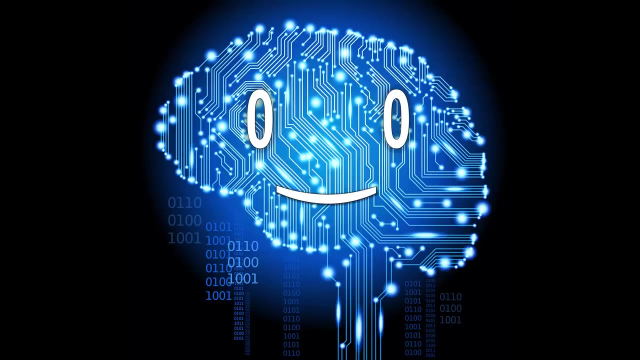 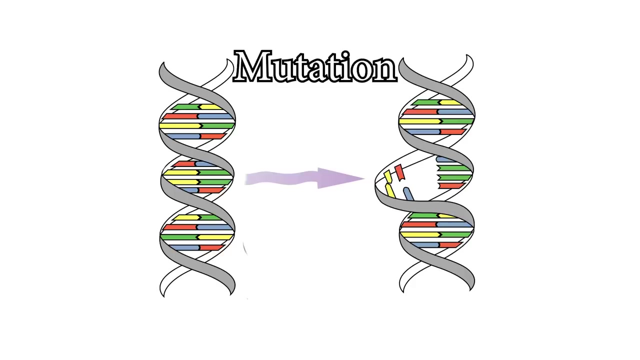 new proteins and dictate how an organism will look like and function After cell division. the DNA is copied in the new cell, But there is a small chance that the replication will not go as planned and some genes will be altered. In this case we have a mutation which is able to change. 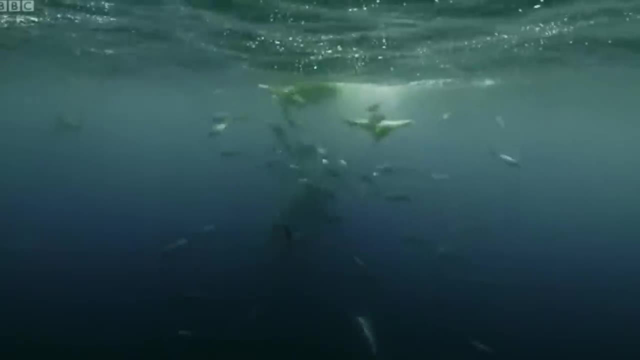 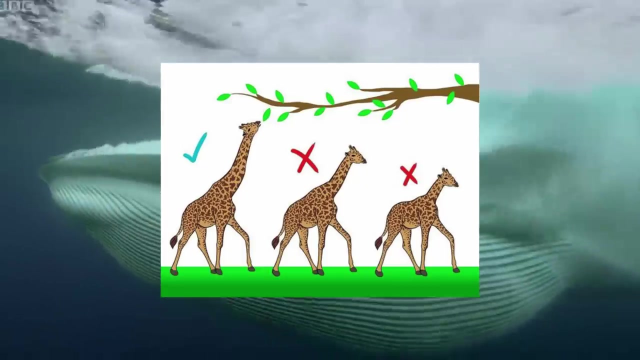 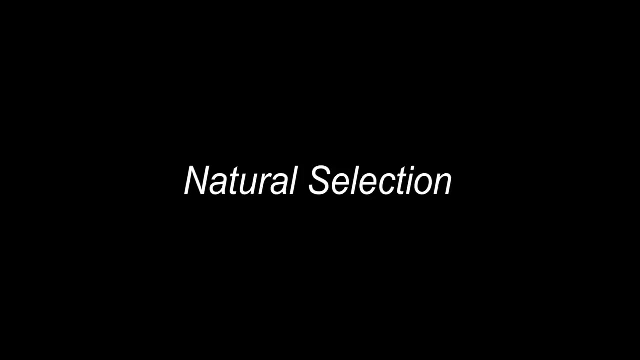 some characteristics of the organism and its offspring. These new traits could be favorable and make the organisms more likely to survive and thus produce more offspring, While specimens with favorable mutations go extinct. This principle is called natural selection, and it constitutes the key mechanism of evolution. And the last one is homeostasis, which represents the ability. 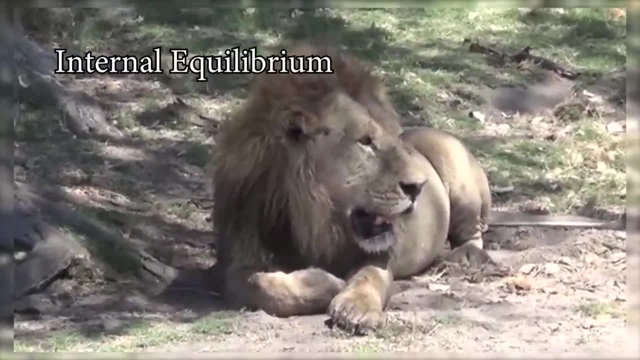 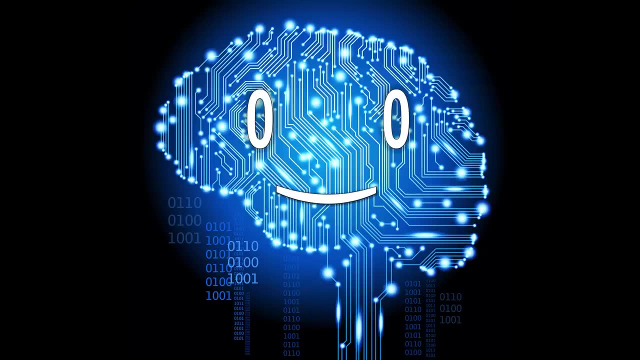 of maintaining a certain equilibrium of physiological processes in living systems for an optimal function of organs and cellular processes. This balance is maintained by many regulatory mechanisms which perceive some perturbations from outside and react to them. For example, if you wear a mask and use it for a long time, you will feel that pressure is there, but 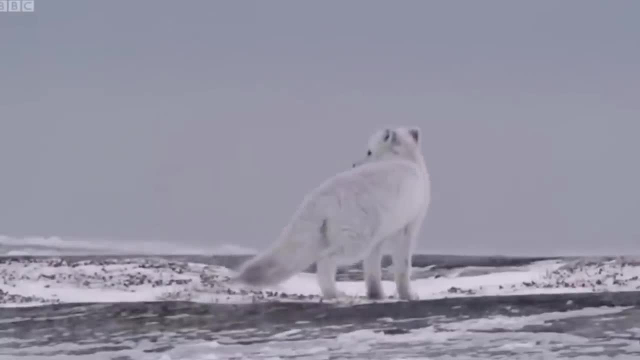 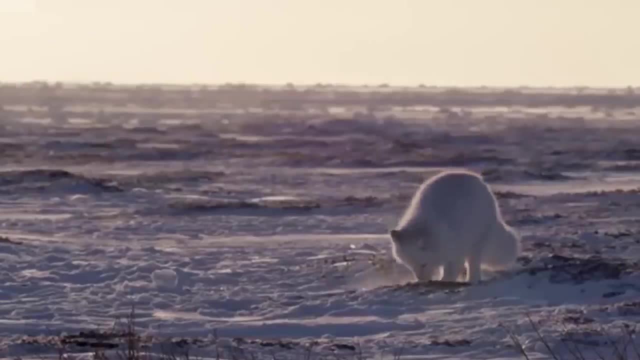 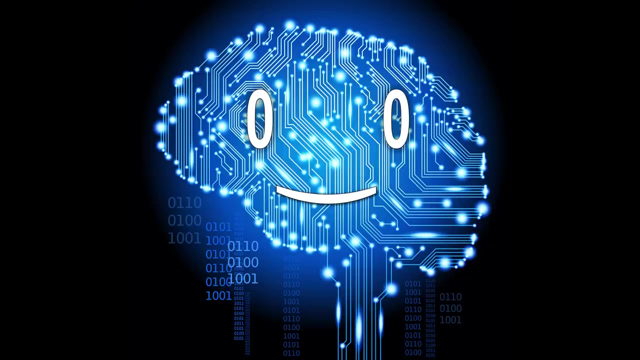 For example, mammals have the ability to regulate their core temperature in response to the low outside temperature in order to keep their organs working and not freeze to borderline death, like how the majority of dumbass amphibians do. For something to be classified as a living being, it must be composed of cells, be able. 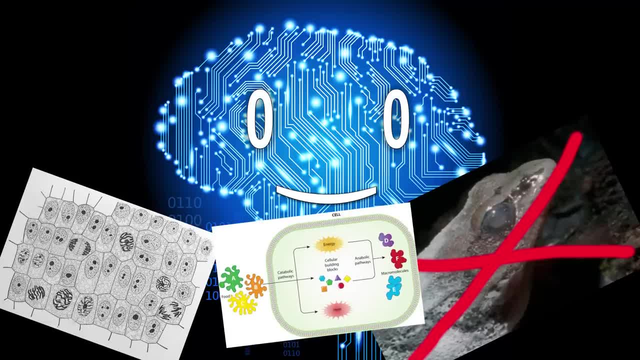 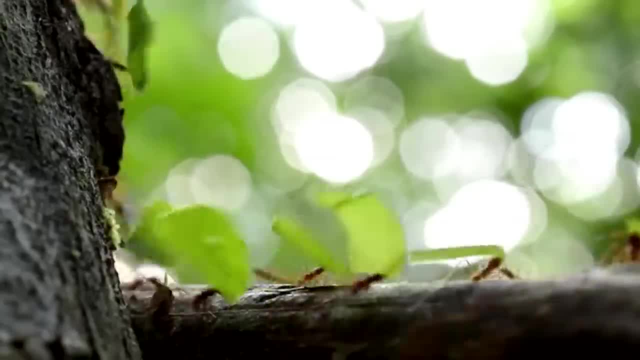 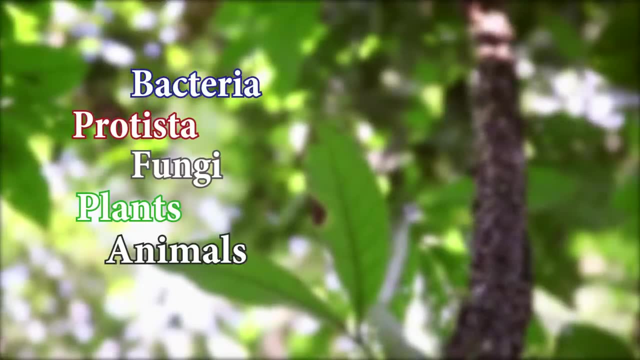 to maintain homeostasis, undergo metabolism, have a life cycle, be able to grow, adapt to the environment and reproduce. The stuff that is considered alive is classified in five kingdoms: bacteria, protista, fungi, plants and animals. There are more systems of classification, but this one is the most popular. 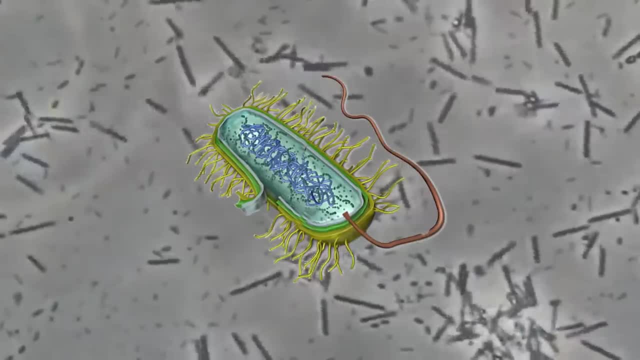 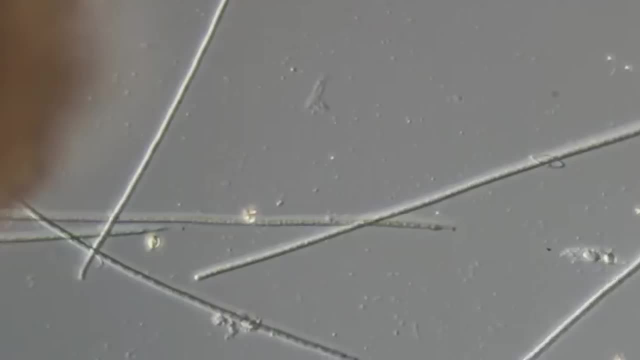 Bacteria are single-celled organisms with a simple internal structure that lack a nucleus and contain DNA that just freely floats inside. They were one of the first forms of life to appear on Earth and thus evolved to live in water, soil, acidic hot springs and even in the air. 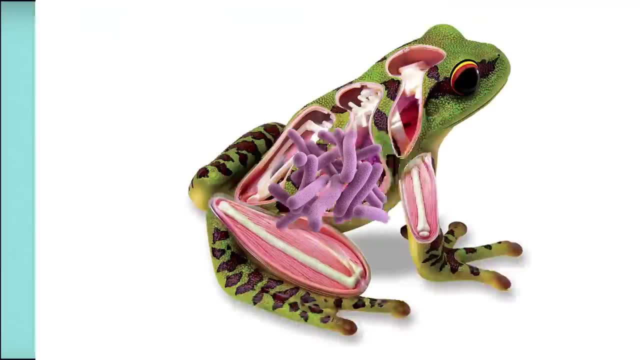 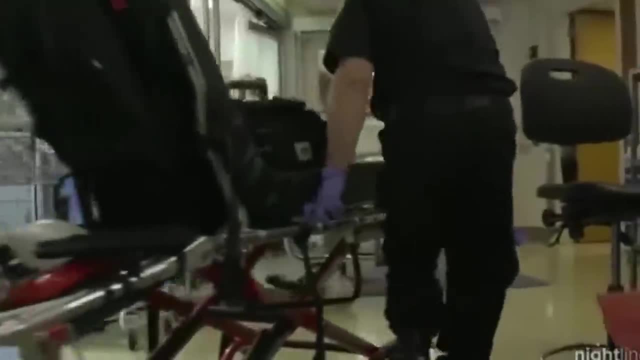 They are also known for their presence in the air. Bacteria are also known for their presence in water, soil, acidic hot springs, radioactive waste and inside other organisms, And while some of them are helpful for digestion, certain species of bacteria are responsible. 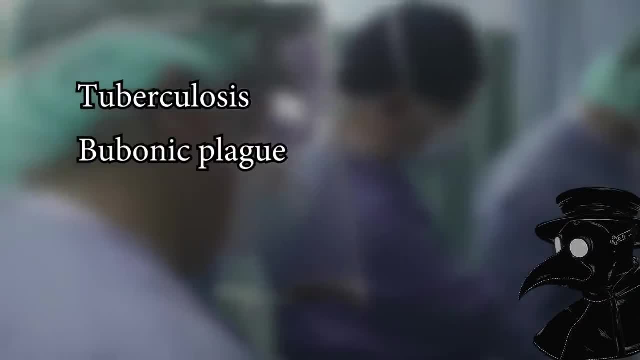 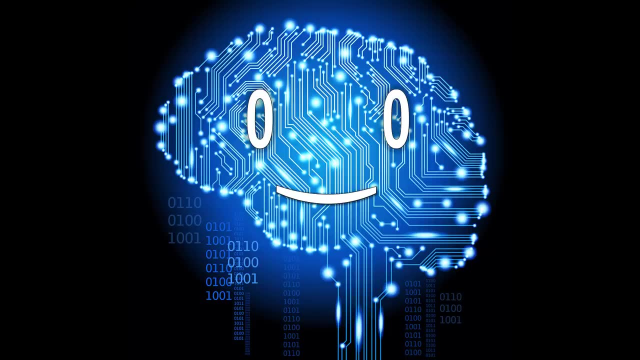 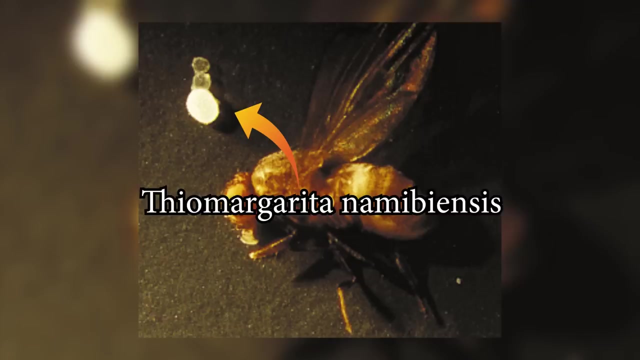 for diseases like tuberculosis or the bubonic plague. Their size typically varies between one and five micrometers in length. However, there are a few species that are visible to the unaided eye, like the Theomargaritonibiensis, which can reach up to a millimetre in size. 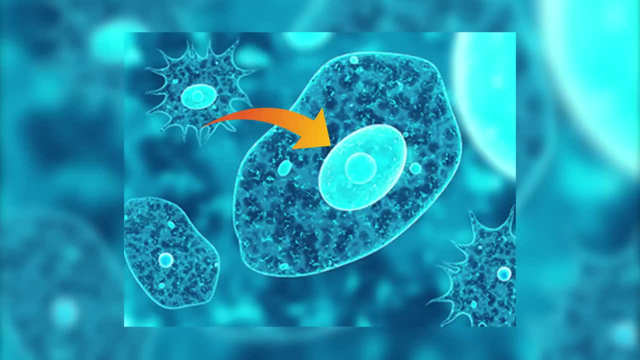 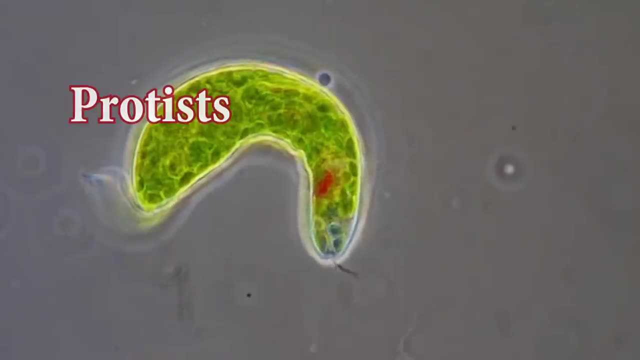 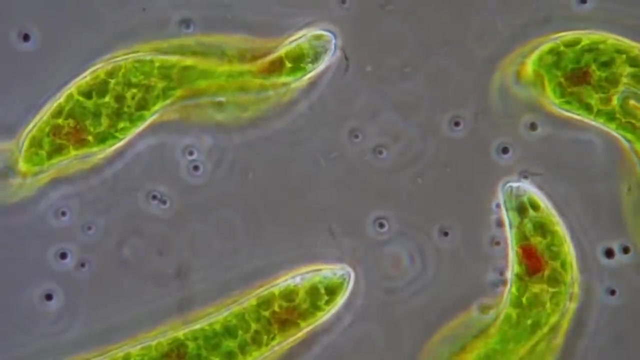 The other types of organisms actually have a nucleus in which they responsibly store their DNA and are called eukaryotes. The most simple eukaryotes are the protists, which is actually a very wide term for every unicellular organisms that have a nucleus and cannot form any tissues. 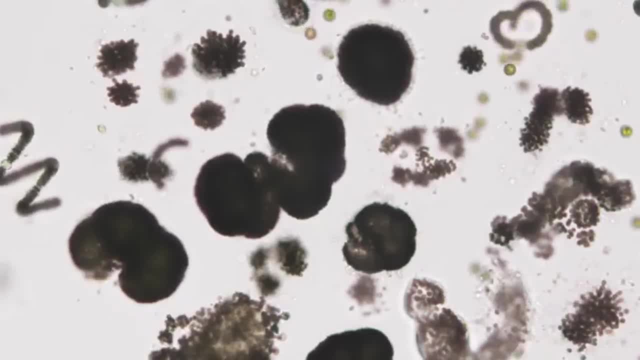 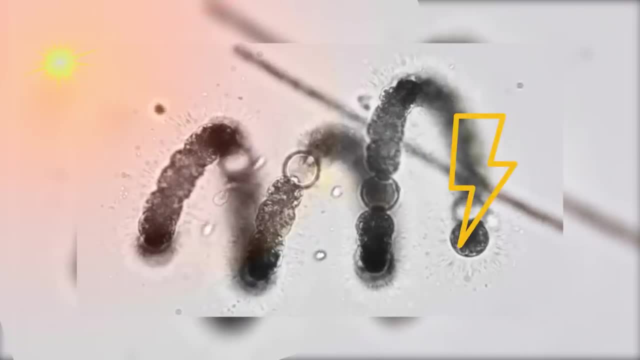 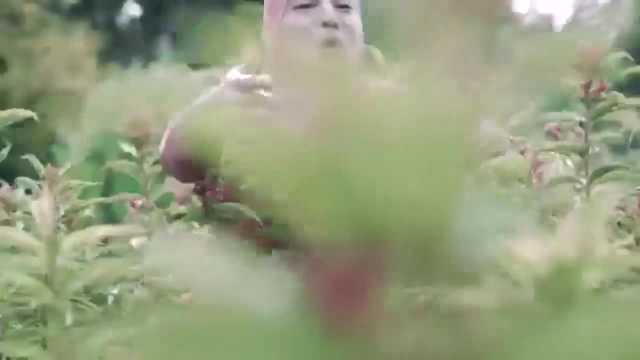 The best they can do is to form colonies and help each other survive, like how the algae do. Eventually, some protista, which were able to turn sunlight into energy, evolved into plants, Multicellular organisms that are able to photosynthesize. I'm sure you've seen a plant at least once in your life. 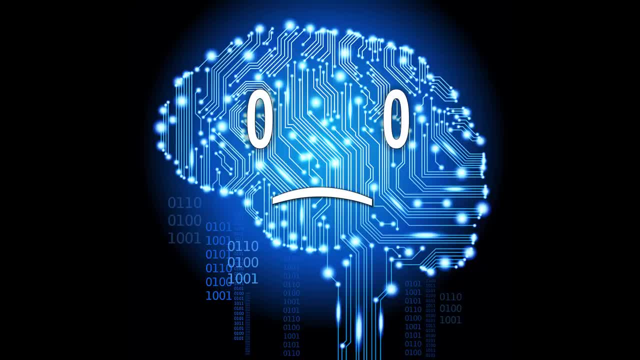 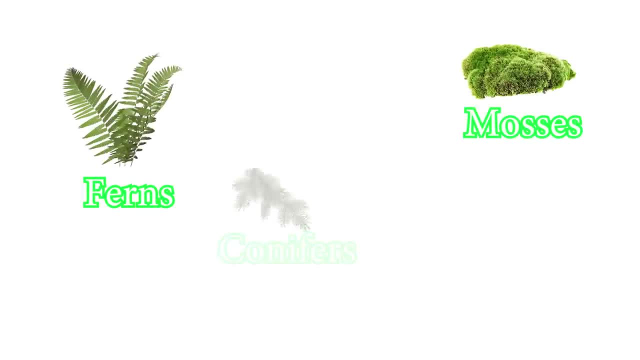 If not, you probably haven't evolved eyes yet. All in all, plants are pretty boring, and I'll just add their classification into ferns, mosses, conifers and flowering plants. Fungi are like the weird cousin of plants and animals. 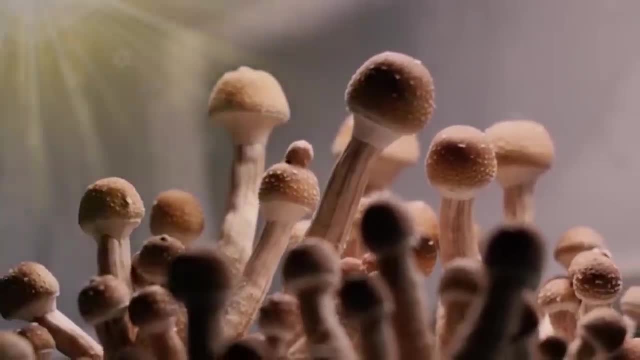 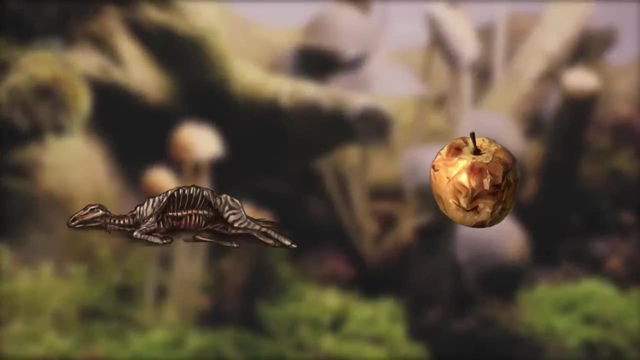 They tend to stay in place like plants, but do not have the ability to photosynthesize. that means they have to get organic carbon from other sources, like plant or animal matter, instead of producing it from anorganic carbon molecules just like animals. 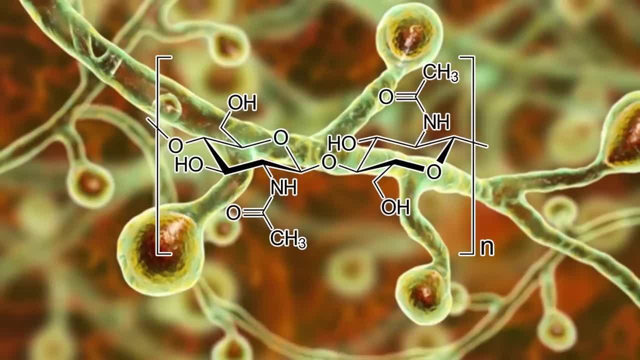 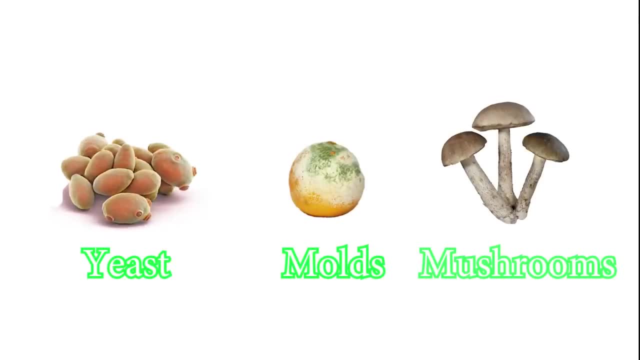 An individual characteristic of fungi is the presence of chitin in their cell walls. This kingdom consists of yeasts, molds and well shrooms, And the last and the most epic one, Animals. For only 46 and 99 evolution points you will get. 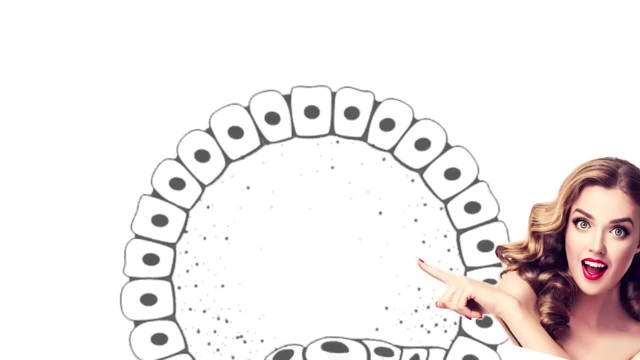 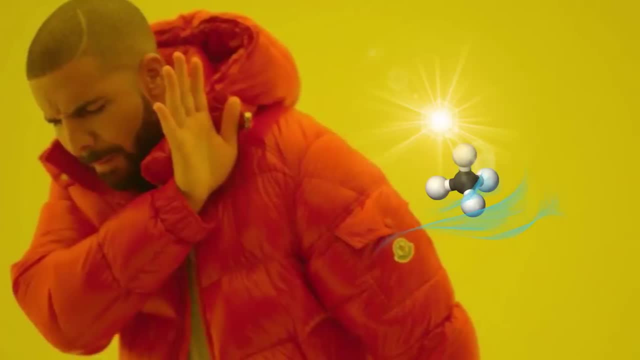 The last and the most epic one: Animals. Get the ability to start your life from a blastula, which will allow you to develop specialized tissue and organs later on in the game. Also forget about producing organic material from anorganic sources like air and light. 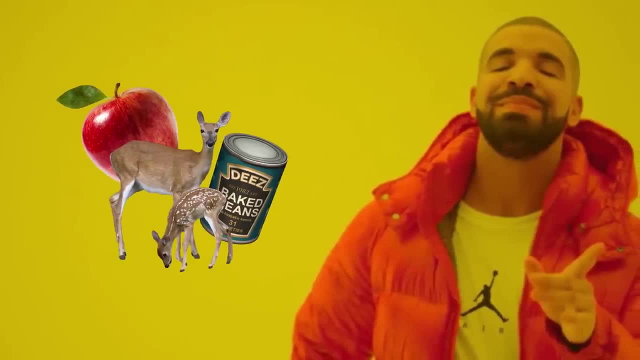 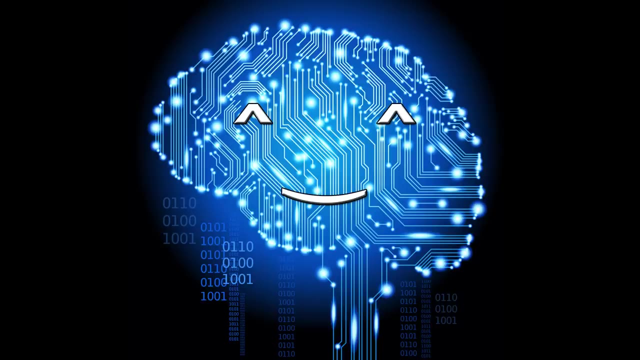